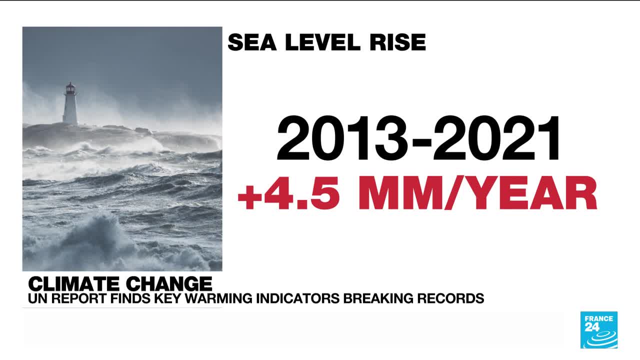 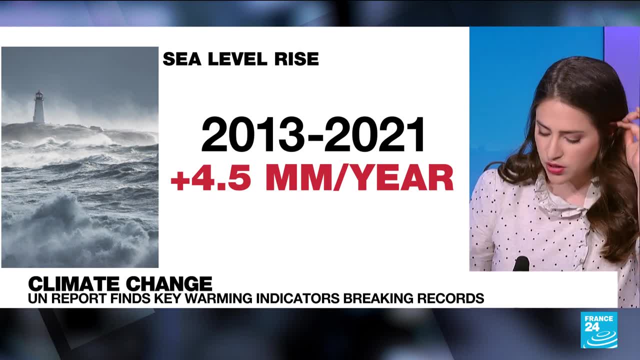 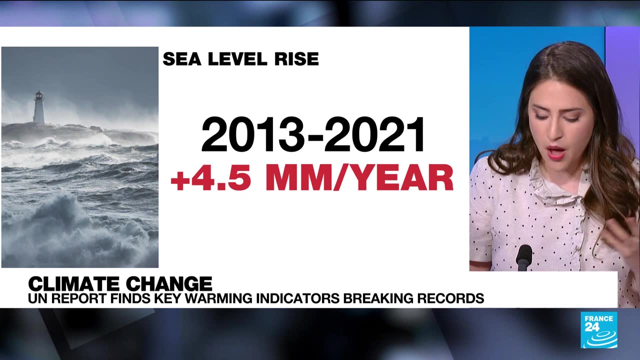 sea levels rose by 4.5 millimeters every year, And if we compare that to that previous period of time between 2002 and 1993 and 2002, we can see that sea levels rose by only 2.1 millimeters per year. Greenhouse gas emissions, of course, are the culprits in all of this. 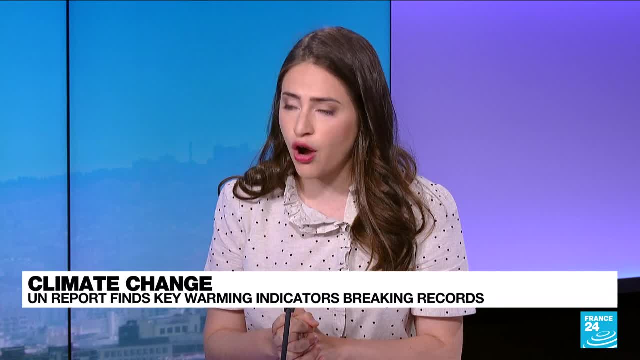 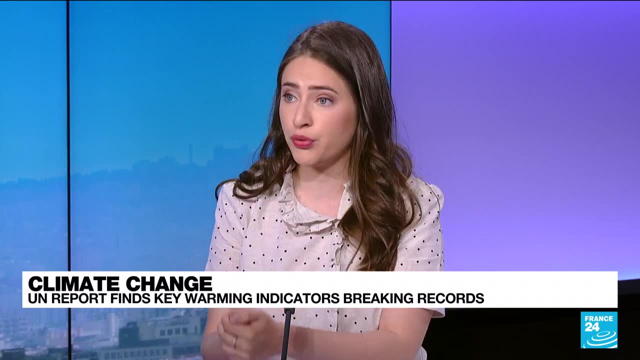 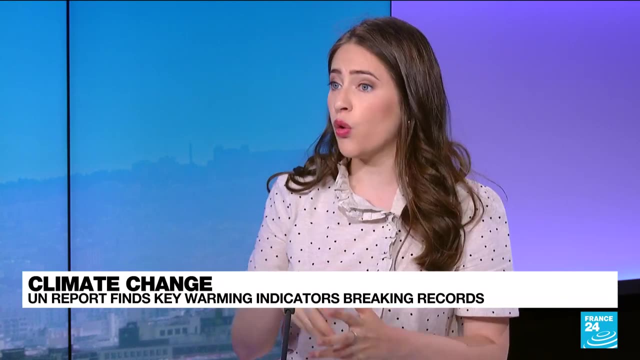 We've also reached new highs in terms of concentrations in the atmosphere, increasing by 150 percent, according to that report, compared to pre-industrial levels. In other words, what does it mean? It means that the degradation of the environment is only getting worse And we 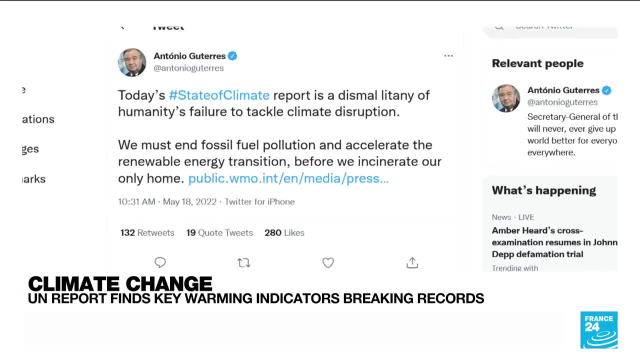 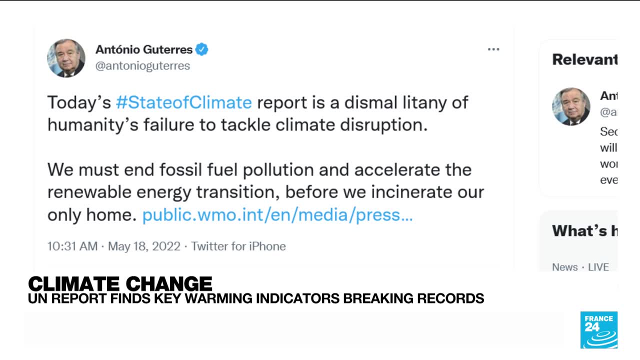 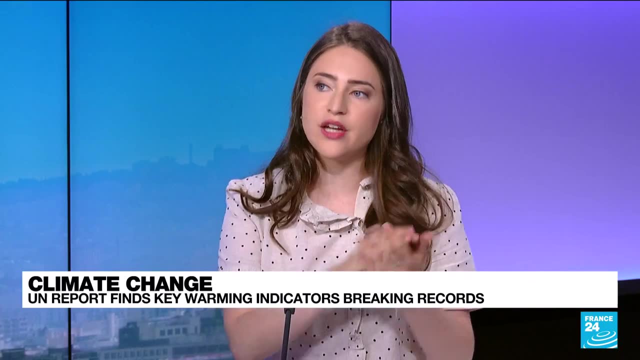 saw a reaction from Antonio Guterres just this morning, who described the report as a dismal litany of humanity's failure to tackle climate disruption, And all of this at a time when we are seeing dramatic heat waves around the world In India. 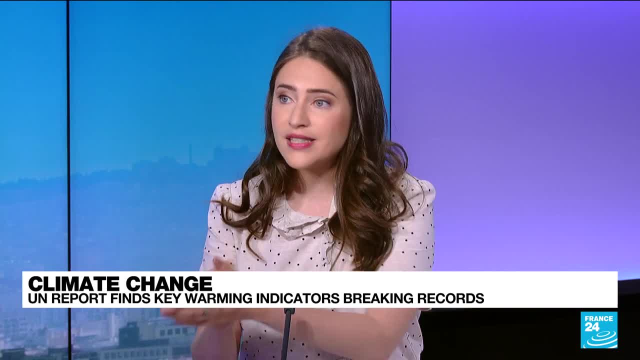 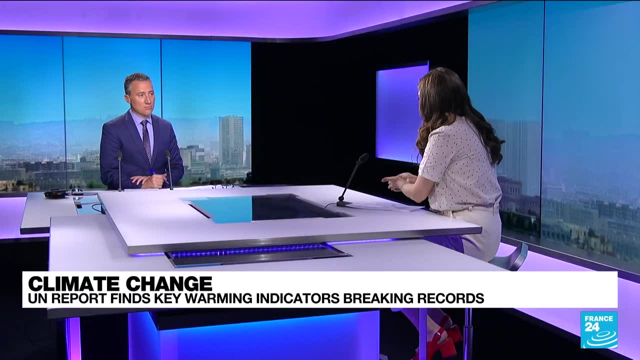 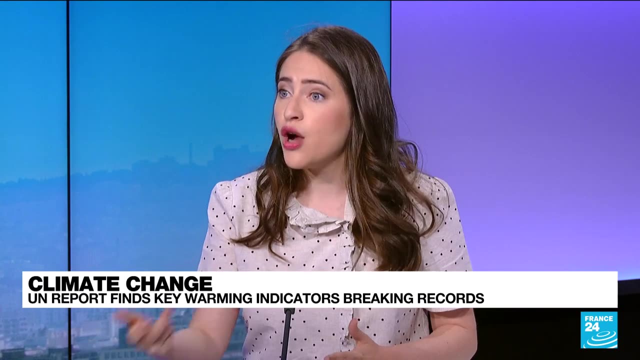 for example, temperatures have reached 50 degrees Celsius. Even here in France- we have seen Monty- we are experiencing temperatures above average, as the spring has only just begun. So I think that perhaps this report will offer yet another reminder to world leaders of the urgency to act, and especially here in France, perhaps, as 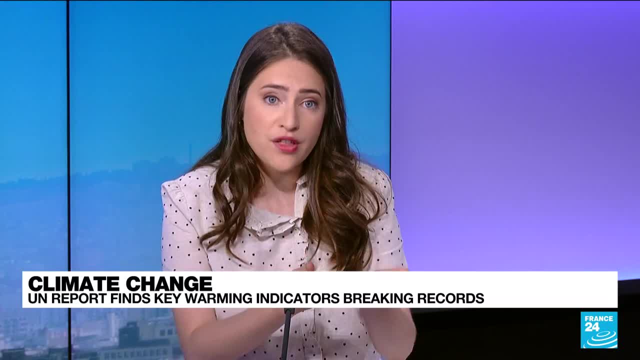 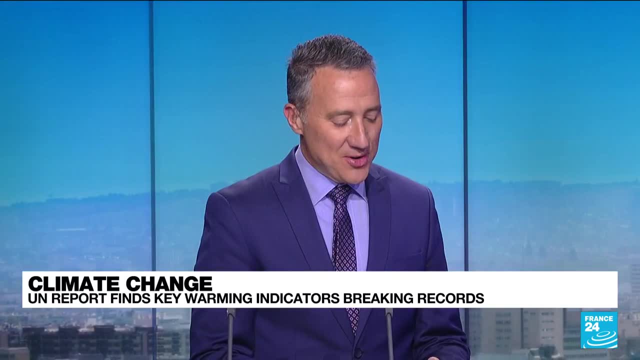 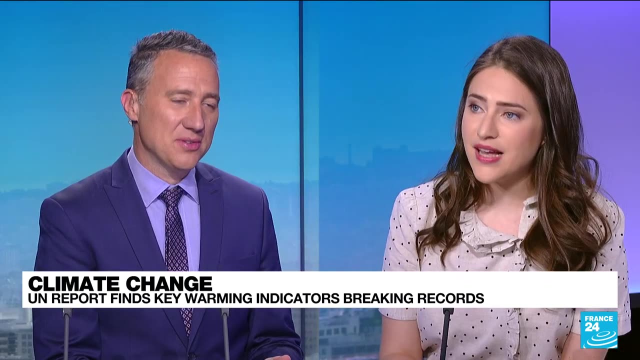 we are expecting a new government to be unveiled with a new prime minister, a new environment minister. excuse me, Yeah, we have the prime minister already. So, Valerie, there's another worrying indicator, separate from this report, about deaths attributed to pollution. Yes, So one in six deaths are caused by pollution. A total of 9 million people died. 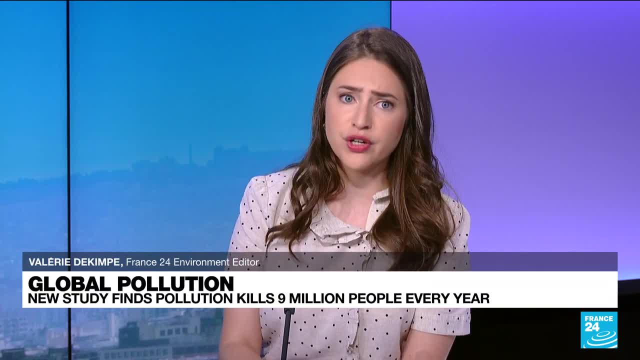 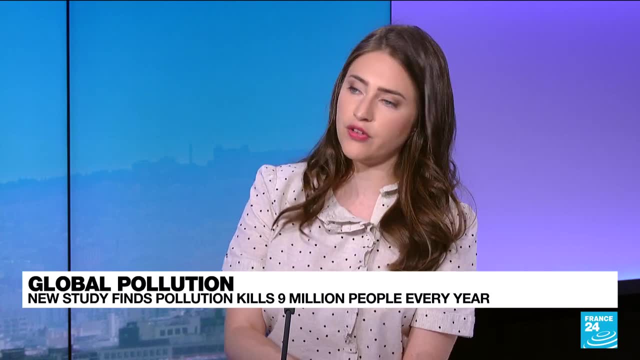 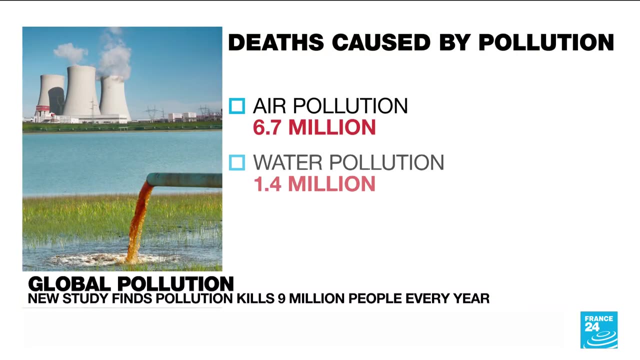 prematurely in 2019 because of various factors related to pollution. That's the conclusion of a report published by the Lancet commission, a scientific journal, today, And let me show you, perhaps, a breakdown of the numbers of what we know from this report: Air pollution killed 6.7 million people, water pollution 1.4 million people and chemical pollution. 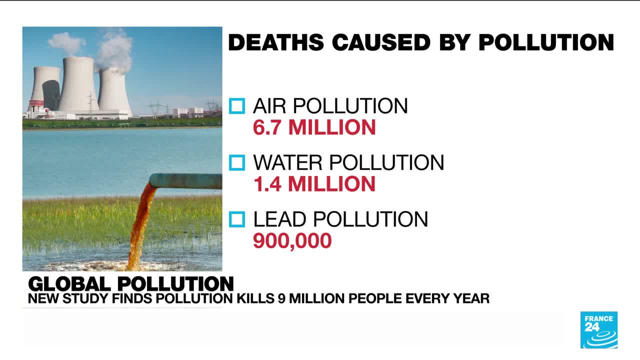 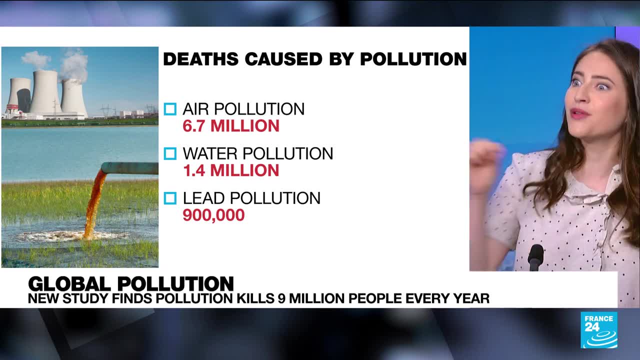 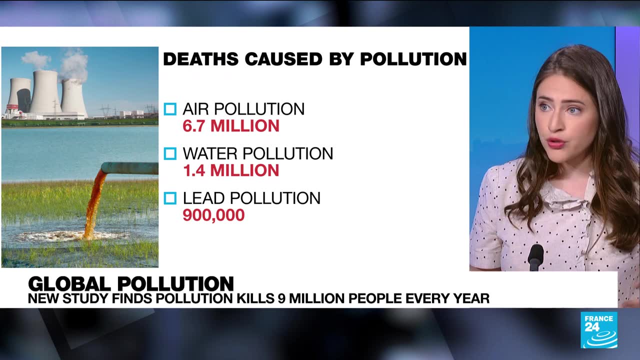 more specifically, lead pollution kills 900,000 people every single year, And what we know is that pollution is a silent killer. It doesn't say pollution on the death certificates, but we know that it causes heart disease, it causes cancer, respiratory problems as well. 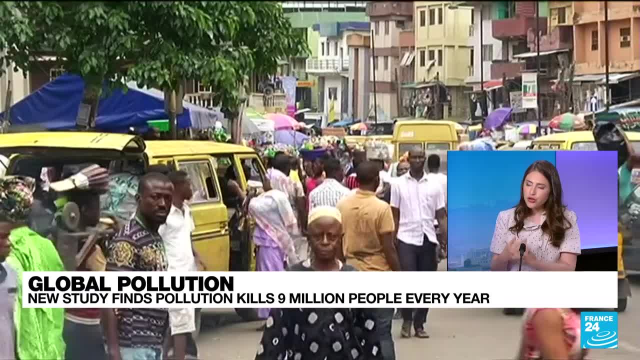 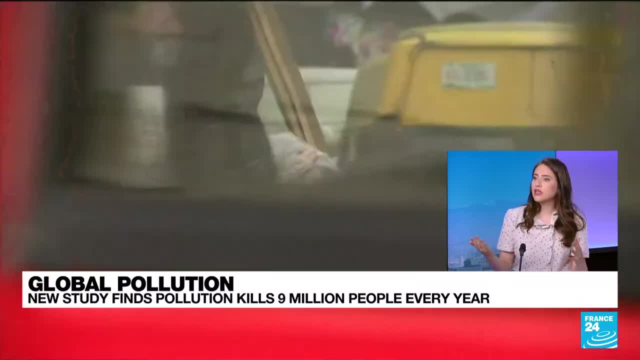 And you also need to keep in mind that the death toll is expected to actually be higher in reality, as the numbers tend to vary. And what's interesting is that researchers the way that they're able to come up with this data is that they combine. 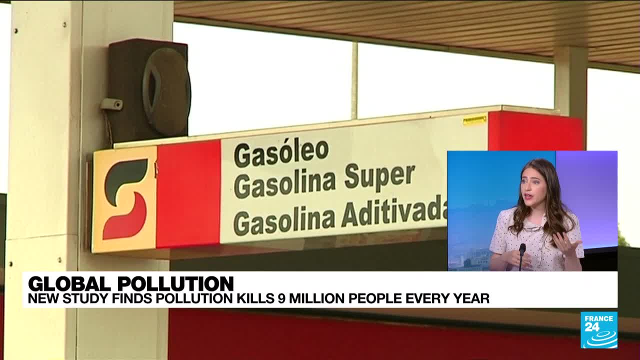 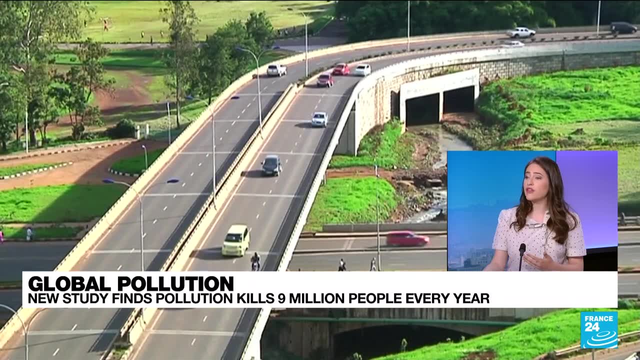 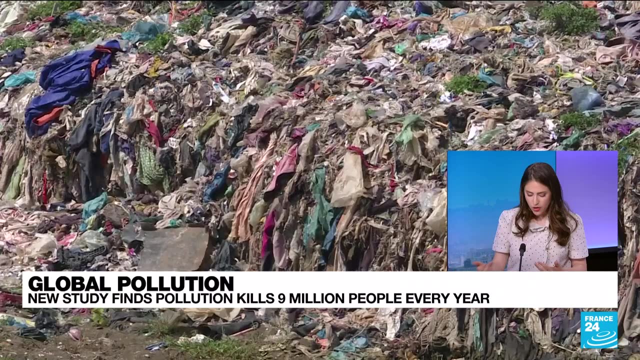 they look at the number of deaths by cause and then they cross-reference that with the likelihood of being exposed to pollution. It's the same way that scientists are able to say to determine the number of deaths caused by smoking cigarettes, for example. 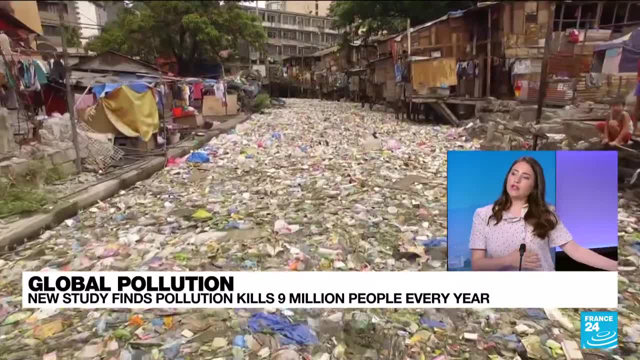 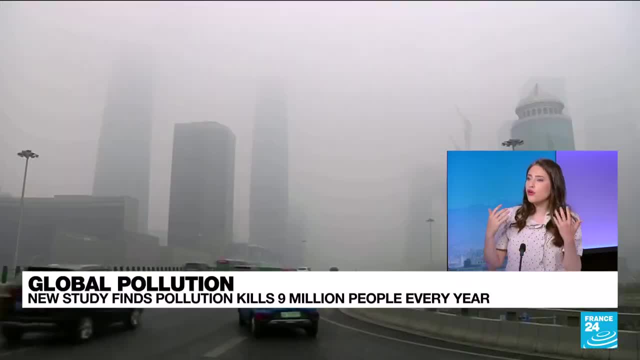 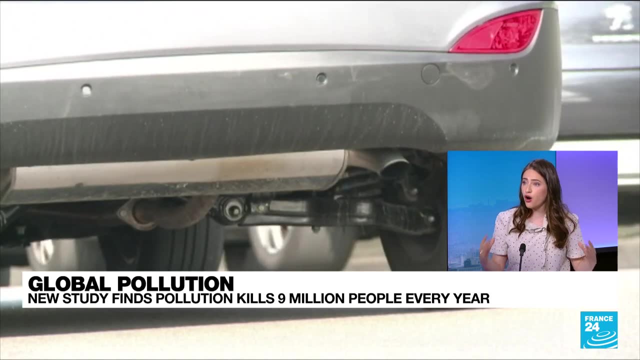 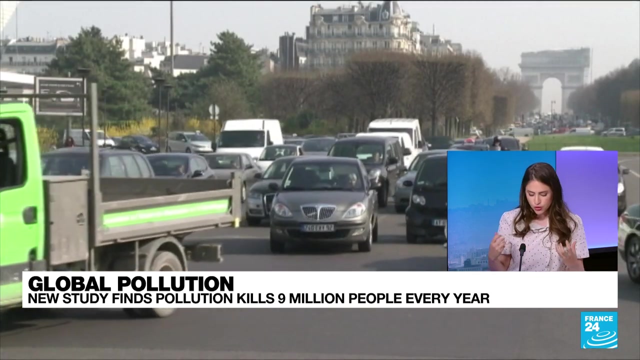 And earlier, just now, we were talking about climate change impacts And pollution deaths are not isolated. They're both closely intertwined. The overwhelming, a huge chunk of pollution, air pollution- deaths are related to coal-fired power plants, to steel mills, to trucks and cars on the roads. 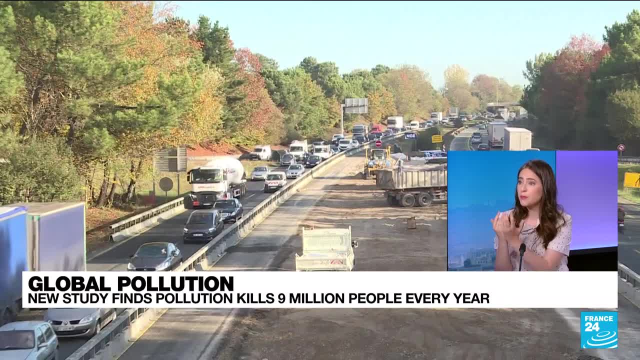 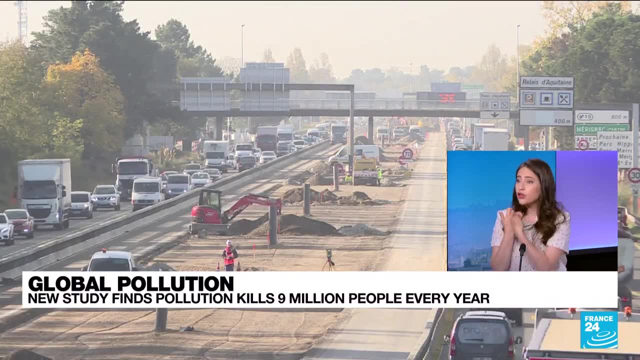 And so both of them are determined by, you know, the fossil fuels that we're burning, the greenhouse gas emissions that we're sending into the atmosphere. So it's becoming increasingly obvious what we need to do in order to tackle both issues. And last thing that I want to say is that we're in a time of crisis. 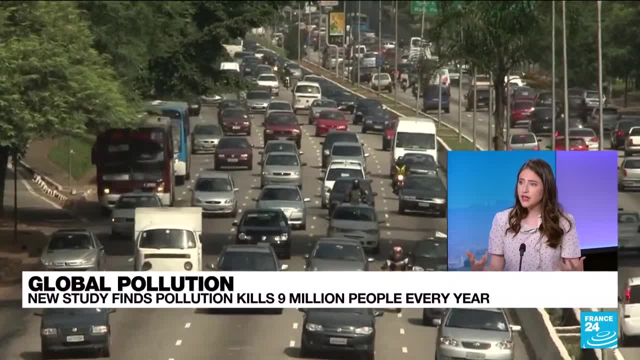 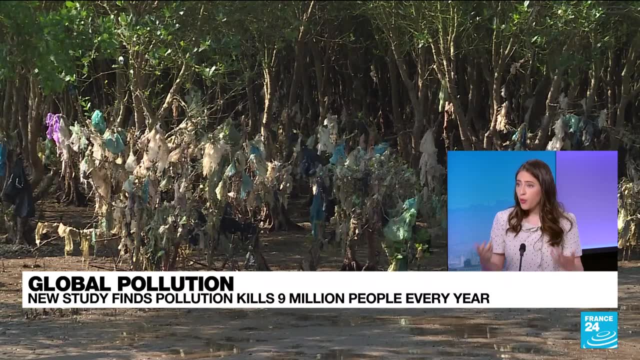 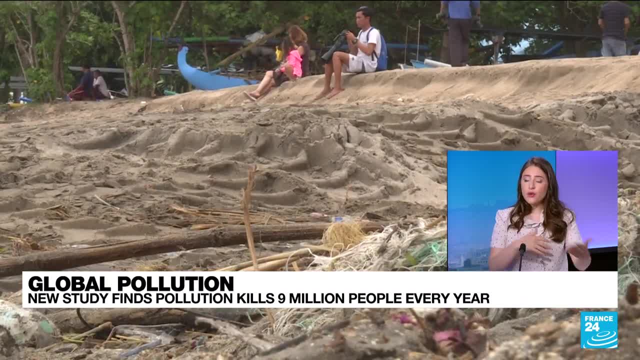 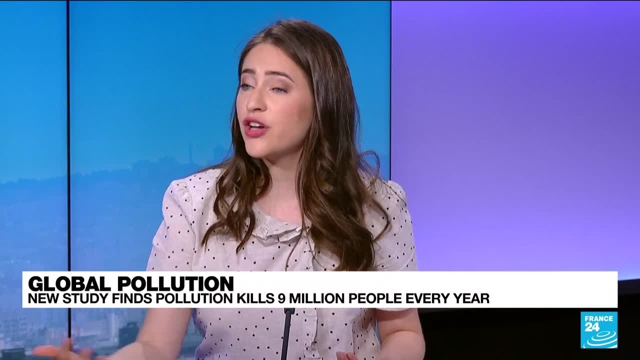 For example, malaria, HIV. now in this report we say 900,000 people died from lead pollution every year. It's more than people who die from HIV every single year and yet it's still undermined and underreported around the world. 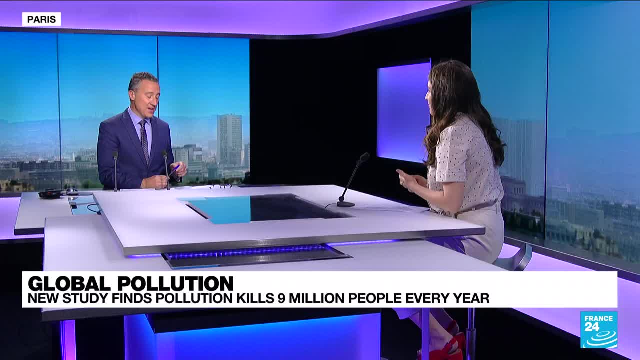 It's more than people who die from HIV every single year, and yet it's still undermined and underreported around the world. Yeah well, troubling news all the way around. Okay, Valerie DeCamp, our environmental editor, thanks a lot. Thanks, Monty.